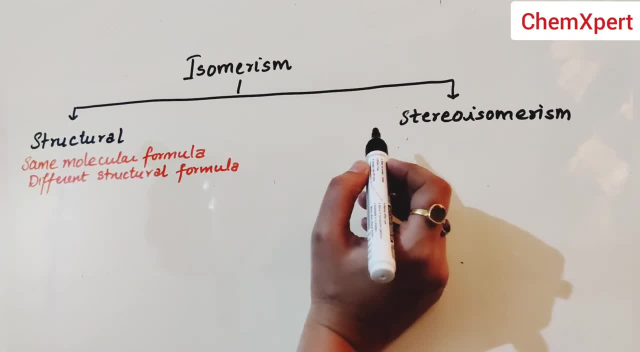 they have a same molecular formula but different orientation in space. as we know, any molecule is a 3D. it can exist in a 3 dimensional figure, so it may possible. their molecular formula is same, but their orientation in space is different, which we will discuss later on. 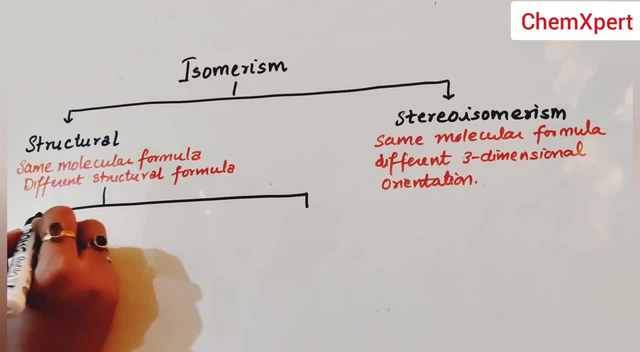 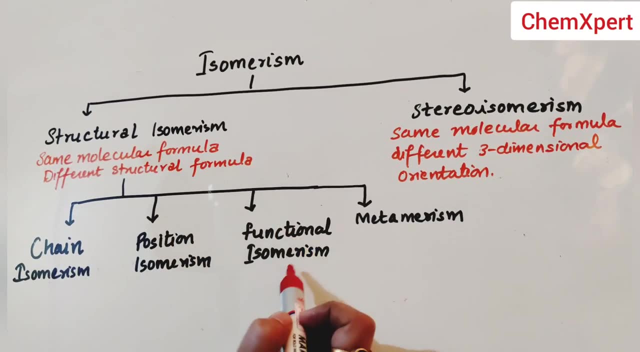 And structural further classified into different section. so these are: chain isomerism, position isomerism, functional and metamerism. Now the chain isomerism is the basic isomerism which you have discussed till now, that is, they having the same molecular formula, same molecular formula but different carbon skeleton. 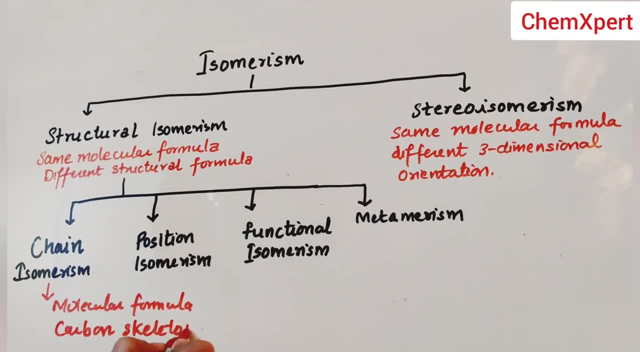 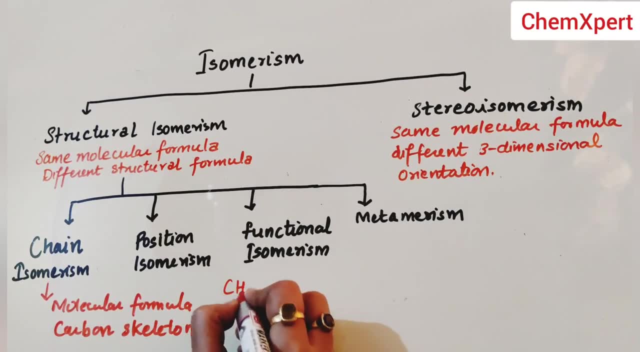 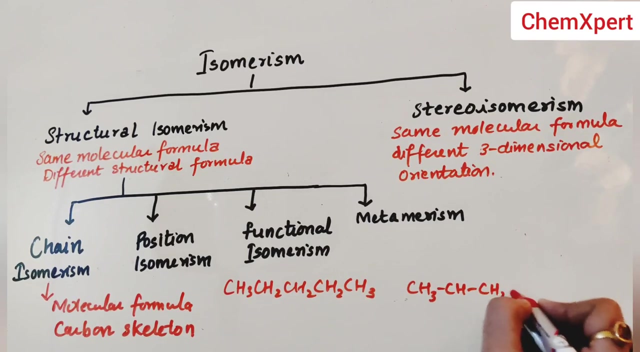 different carbon skeleton. Now, for example, the similar example we will discuss again- for example, pentane, CH3, CH2, CH2, CH2 and CH3. this is the one isomer. the second isomer which can possible for this is this, where we take the four carbon skeleton and make it a branch like this, and the third: 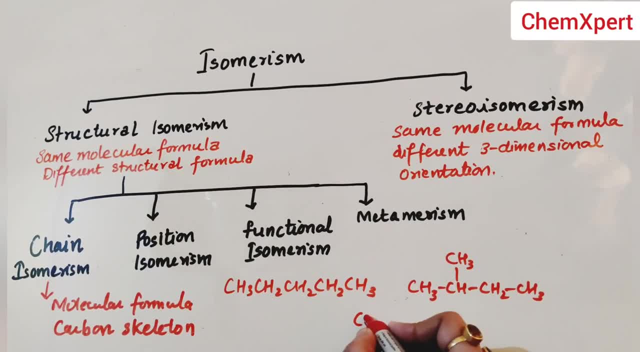 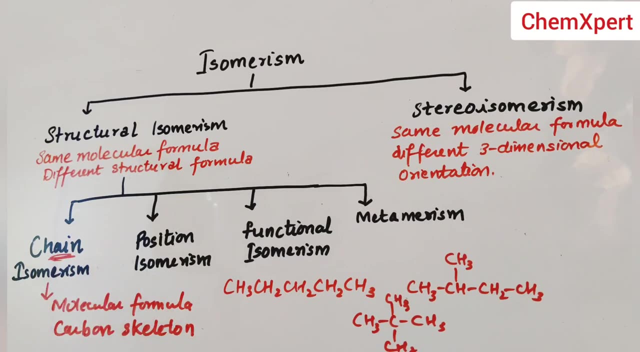 one. This is the three carbon skeleton: CH3 C, CH3 3, then 4, then 5. so these three are the isomer of the pentane, but they are regarded as a chain isomer. why? because there is only difference in the chain length. it is of 5 carbon, it is of 4 carbon and it is of 3 carbon. 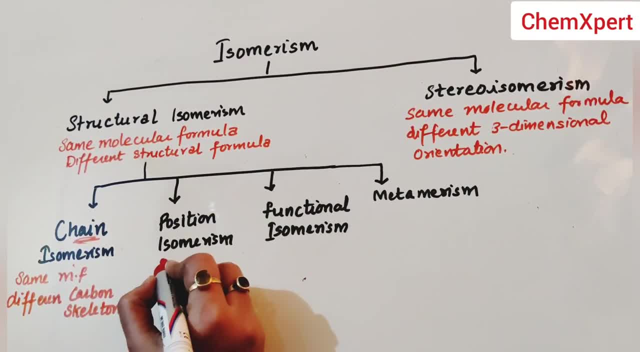 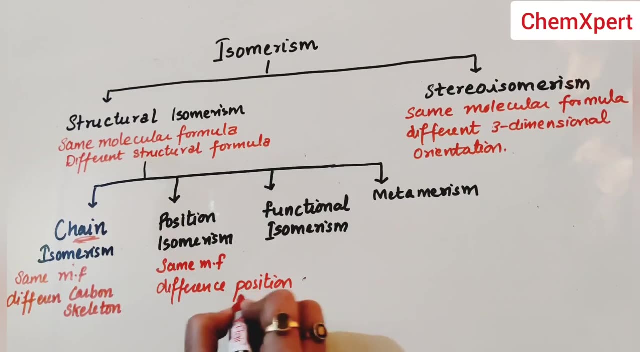 Now next one is the position isomerism, Which again is the same molecular formula, same number of length of the carbon chain, but difference in the position of main point is difference in the position of a substituent. Now, for example, if we draw this but one in: 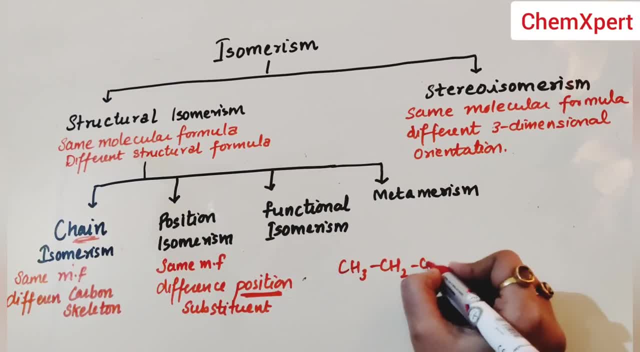 It is CH3, CH2, CH3.. So this is the position of the substituent. Now, for example, if we draw this but one in, It is CH3, CH3, CH3, CH2, CH3, CH3, CH3, CH3, CH2. this is but one in, but when it is position shifted. 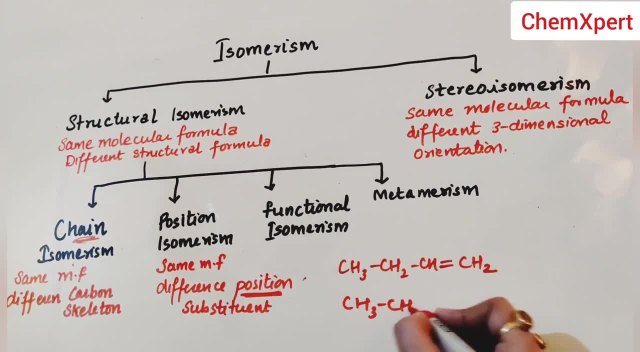 to second one. now again, the carbon length is of 4 carbon, but the position of double bond shifted. This is but one in and this is but two in. So this is known as a position isomerism, because they have the same molecular formula but difference. 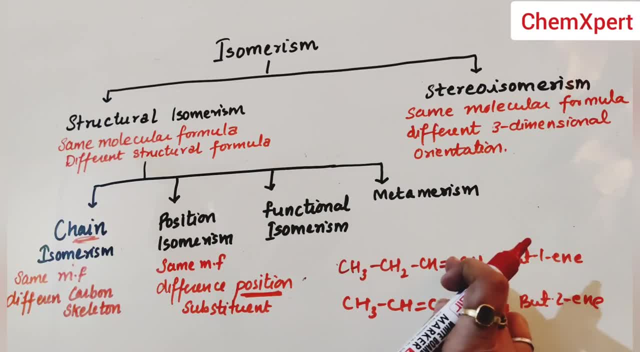 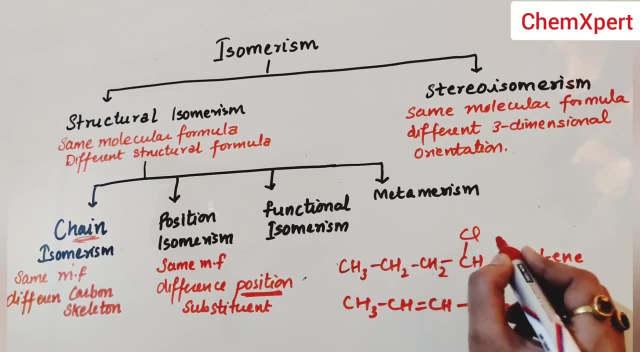 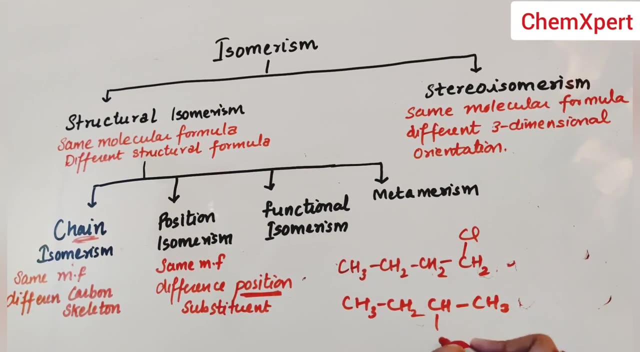 in the position of substituent: substituent. This same example can be for this section. like CH2, then CH2Cl. This is 1 chlorobutane, 1 chlorobutane, and the similar way. if we place Cl at the second position now, it become 2. 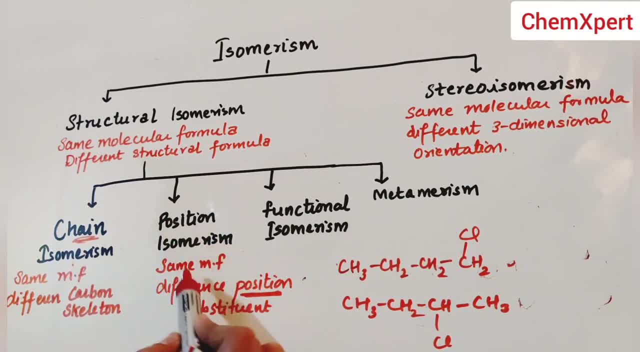 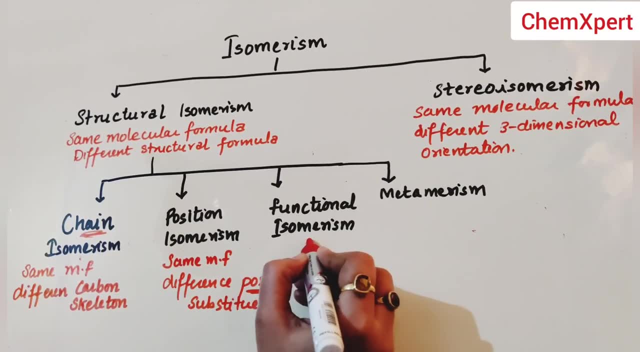 chlorobutane. So again, these two are the position isomers. Next one is the functional isomerism. Again same molecular formula but different functional group present in it, Different functional group. In the last video we have discussed what are the functional group. 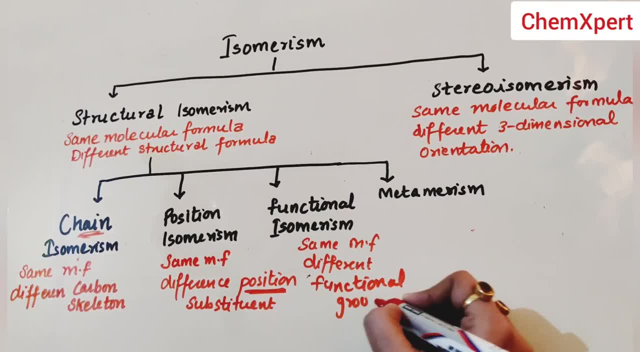 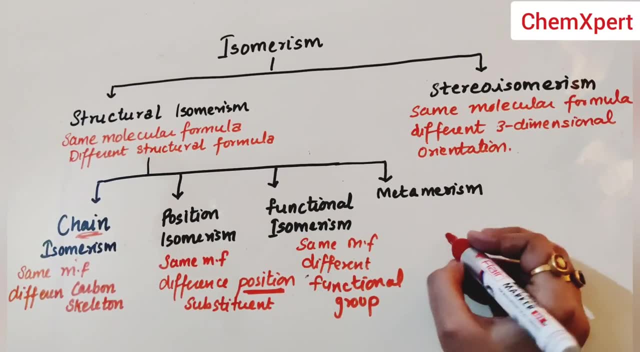 which give the properties to the chemical properties to any of the compound. So, for example, one of the most common one is the aldehyde and the ketone. So imagine 3 carbon aldehyde, that is CH3, CH2Cl. This is an aldehyde that is propanol, having molecular formula C3H6O. Now if we write the 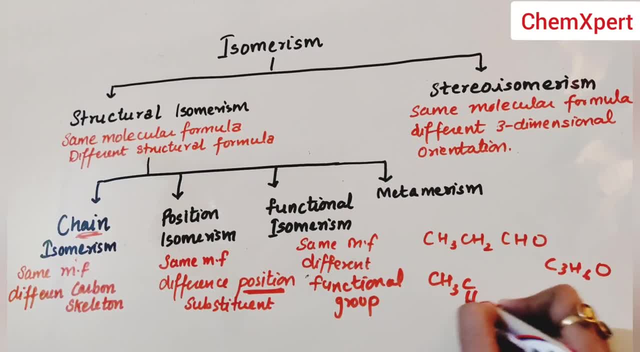 ketone form of this, then it will be CH3COCH3.. So again 1,2,3.. 3 carbon, 6 hydrogen, 1 oxygen. So aldehyde and ketone are the functional isomers. One more example is the aldehyde. 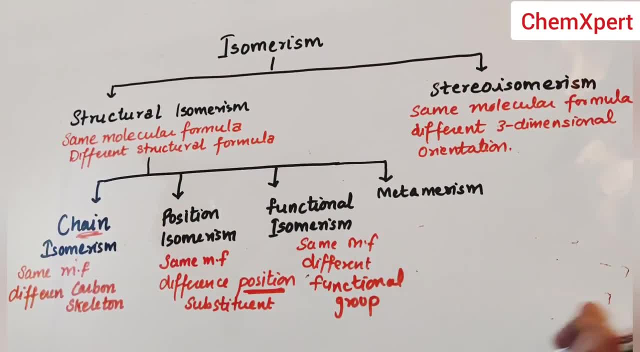 and the TH3H7, this is the hexane combination of 2 and 3.. So look at this. Are these the hom lipstick andмо isto hmm ço. 2 H7.. 2 CH1.. 2 H6.. 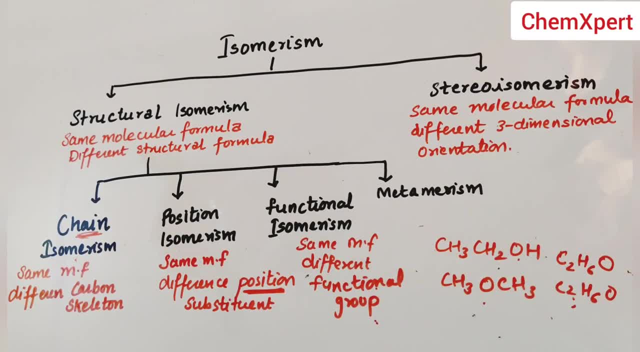 2 CH councils, 2 CH2.. other one contain ether and their properties altogether change because in case of alcohol they have high boiling point because of hydrogen bonding and ether easily evaporate reason: no hydrogen bonding can possible in this case. so they are the functional isomers having the same 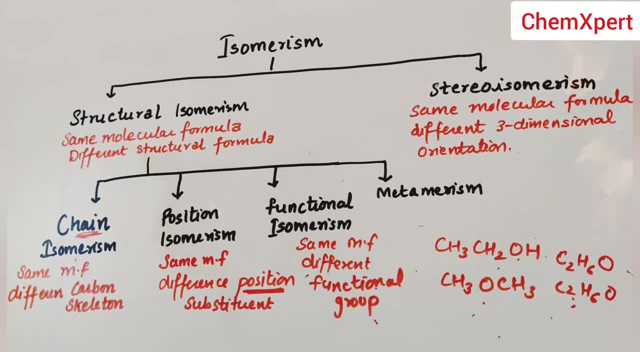 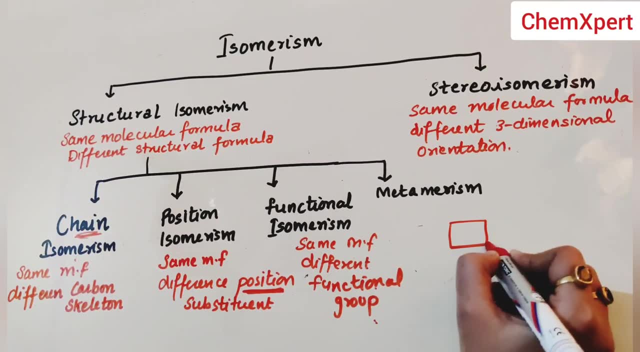 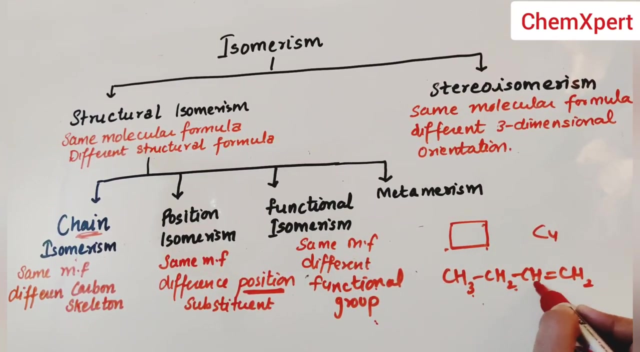 molecular formula, but different functional group. now one more example of functional isomer is these two category. this is cyclobutane, and if we just write simple formula of butane, so again for carbon: 1, 2, 3, 4, C, 4, H, 3, 3, 6, 7, 8, 2 to 4 to 6 to 8, C, 4, H, 8. so general formula is C and H, 2, 1 in both the case. 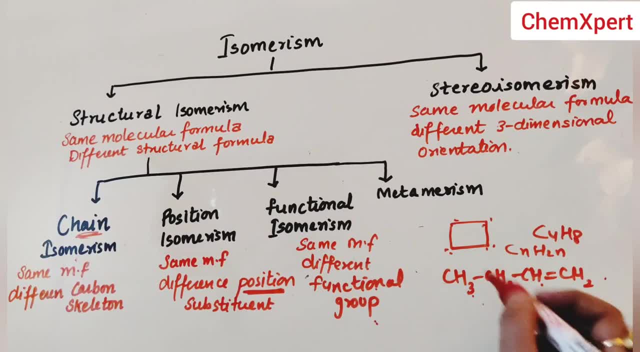 in the cycloalkane as well as in the alkene, but functional group is different in this case: no double. molecular isomer is present in the cycloalkane as well as in the alkyne, but functional group is different in this case: no double. 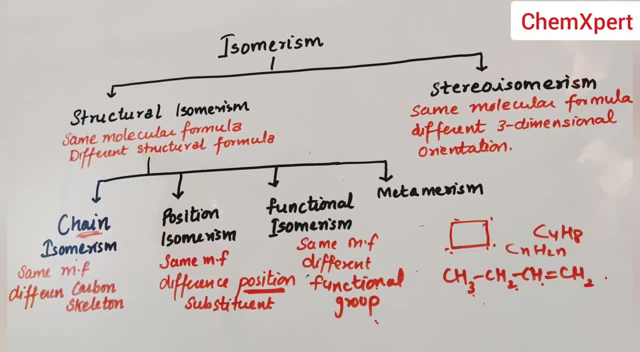 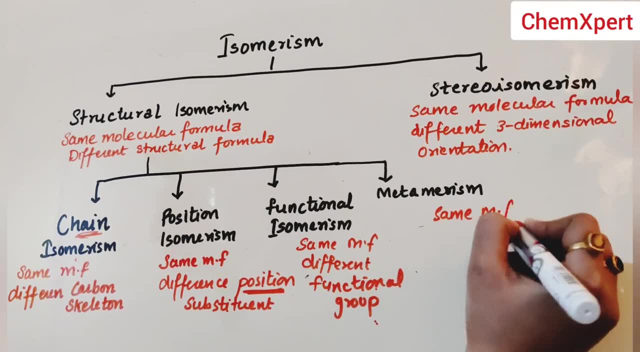 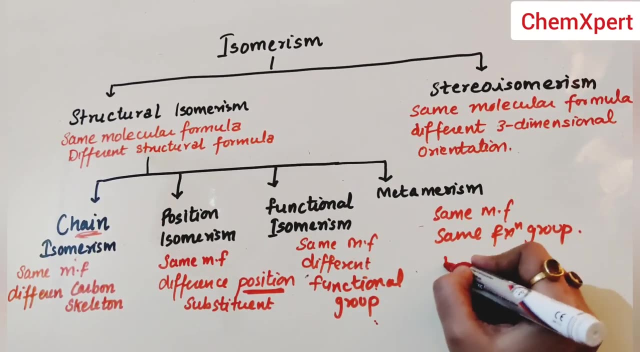 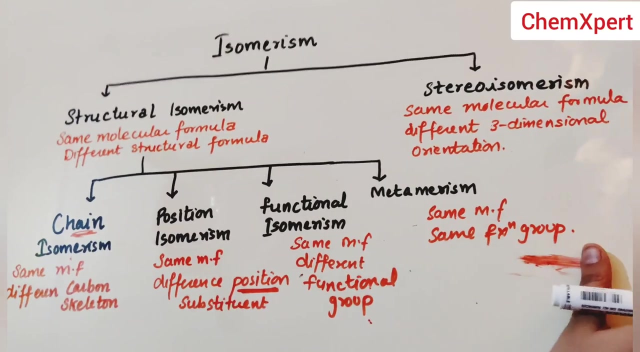 bond is present here, double bond is present now. the metamerism meaning having the same molecular formula, same molecular formula, same functional group also. same functional group also, but the methyl group surrounding methyl group, surrounding that functional group changes. now, for example, in case of ether, ether of four carbon. 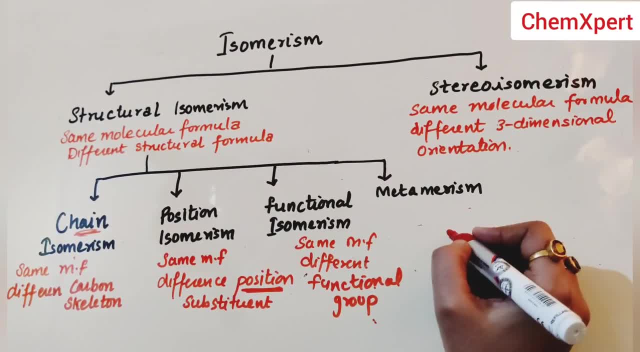 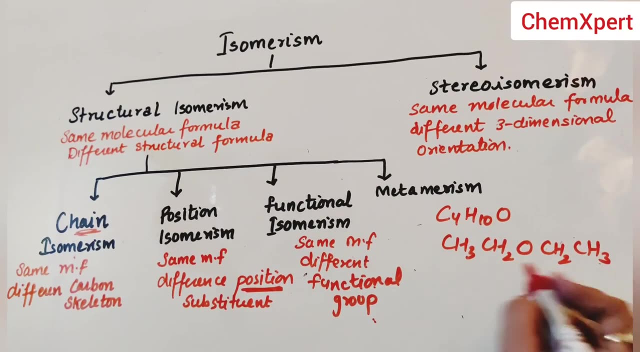 four carbon. ether has a general formula: C 4, H 10 O, C 4- H- 10 O. now we have to prepare ether from these four carbon. it can possible CH3, CH2 O, CH2, CH3. so it is almost one, two, three, four, five, five. 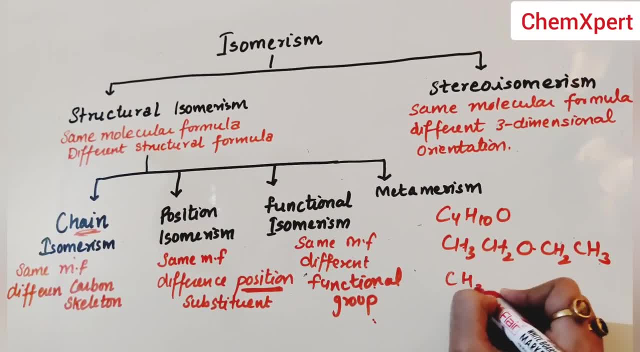 in a chain like structure, but it can also be possible like this. so these two ether are having the same molecular formula, same functional group, that is, ether present in it, but the methyl group surrounding this ethereal oxygen is different, in this case one methyl and one propyl, whereas in this 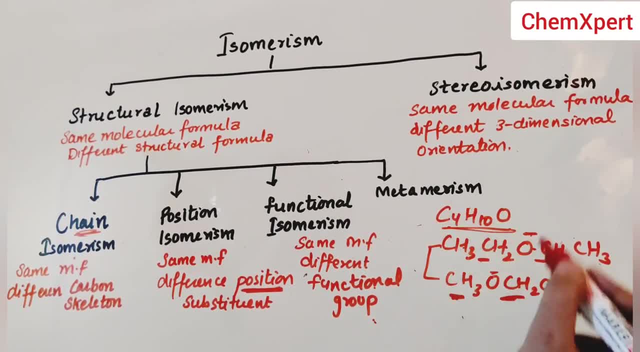 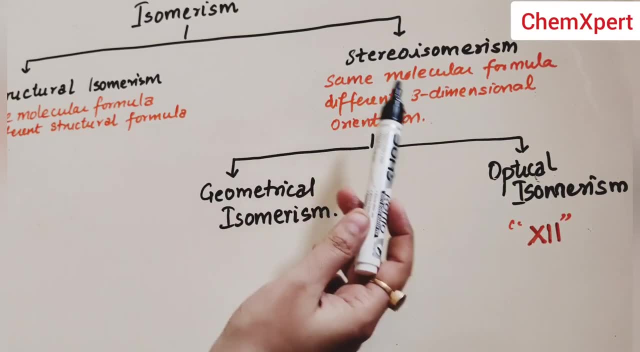 case two ethyl group are surrounded by this. so this kind of isomerism is known as metamerism. now the next classification is stereo isomerism. it is of two types: geometrical isomerism and the optical isomerism. optical isomerism- you 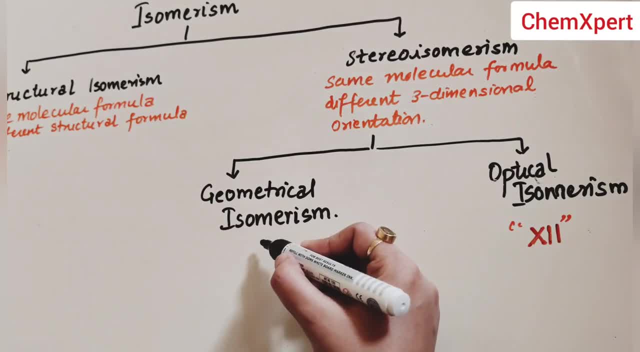 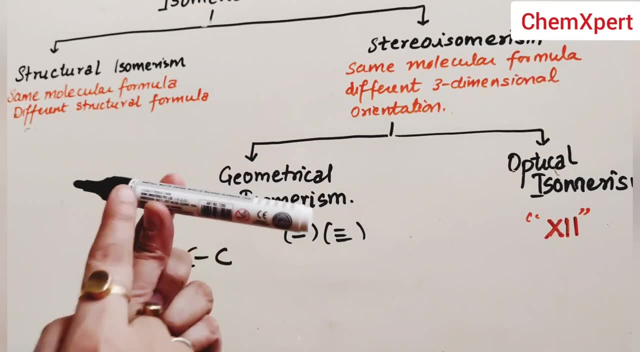 will going to study in class 12, so we will discuss only about the geometrical isomerism. for example, whenever there is a single bond between two carbon, it is just like this: a single bond and there at the two end, two carbon is there, so there is a free rotation around. the bond is. 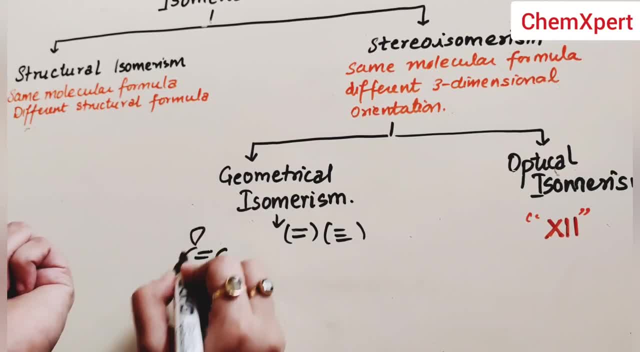 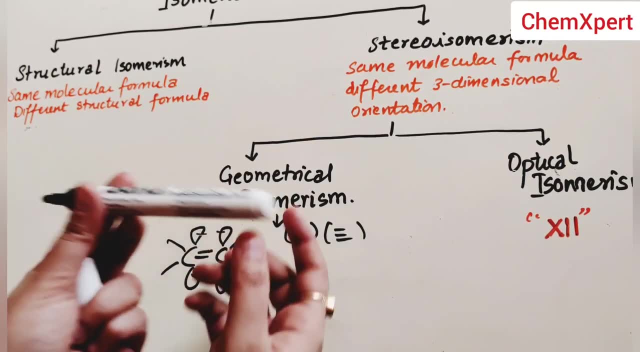 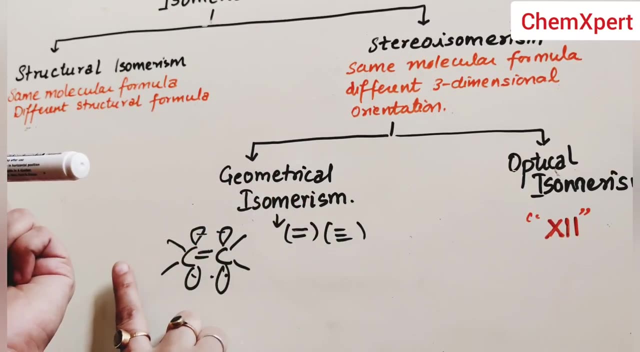 possible. but when it is a double bond, meaning the bond which is formed by the PP overlap, this is a single bond. so now, because of this overlapping, now this bond is not in a free rotation around the carbon atom, so now we cannot rotate it, otherwise, until it was a single carbon. 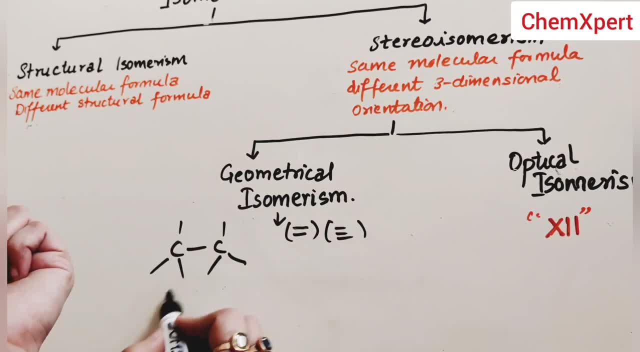 single bond like this is a position, so we can rotate and reverse this position, because rotation is possible around the single bond, but when it is a double bond, rotation is not possible. this is a simple ethylene molecule. so what happened in ethylene? all the atoms of the end are the same. 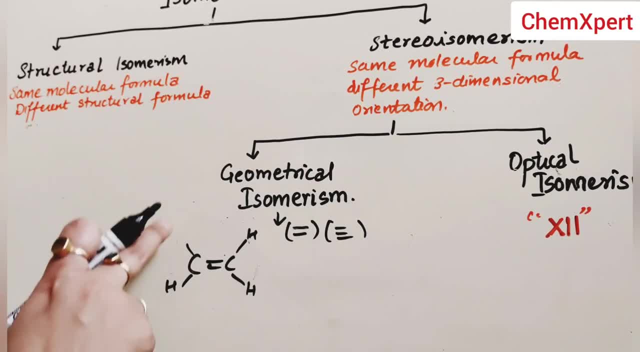 now if, instead of these atoms, I did but-to-ine? but-to-ine means there is CH3 at one end and CH3 at the other end. also, there is a chain of four carbon: one, two, three, four. so it is but-to-ine now. 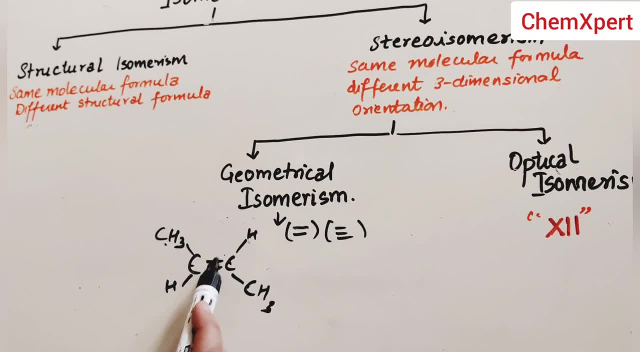 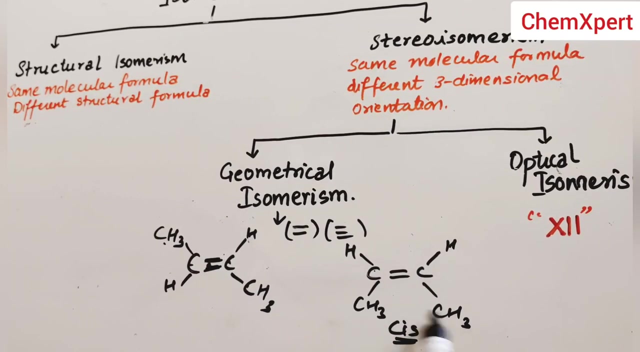 the possibility is that if you are around this double bond, these two alkyl groups are present diagonally and there can be one more arrangement of this only. and there can be one more arrangement of this only when these methyl group at the same side. so these are the two form or geometrical isomer, one is known as the cis, when the group are on the